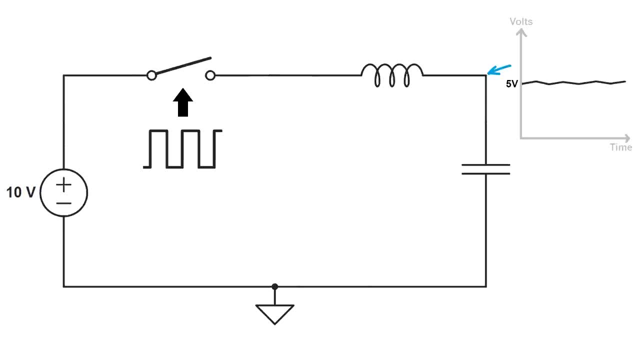 Now let's add an LC low pass filter. The inductor resists sudden changes in current and the capacitor resists sudden changes in voltage. The combined effect is that our LC low-pass filter averages out the square wave and we get 5 volts of relatively steady DC on the output. 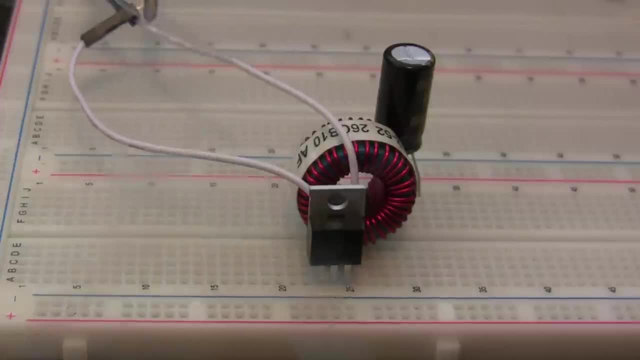 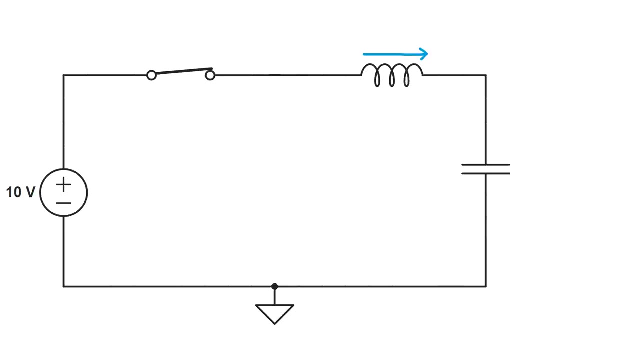 Now, unfortunately, if you build this in real life, this'll happen, but why? Well, let's say the switch is closed and our power supply is delivering some current. This means that current is flowing through this inductor. Now let's open the switch. 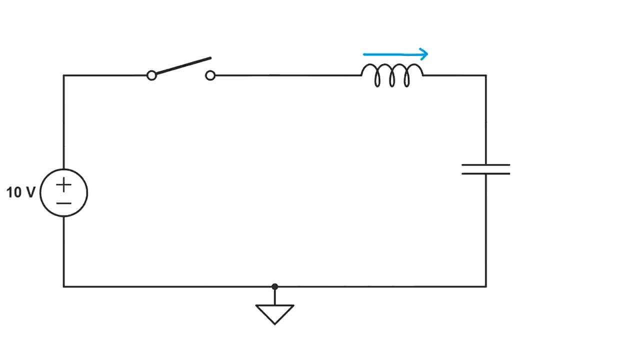 Since current in an inductor cannot instantly change, this means that current is still flowing through the inductor, but this side of the inductor isn't connected to anything. So you get this huge mass of electrons building up here, creating a massive negative voltage. 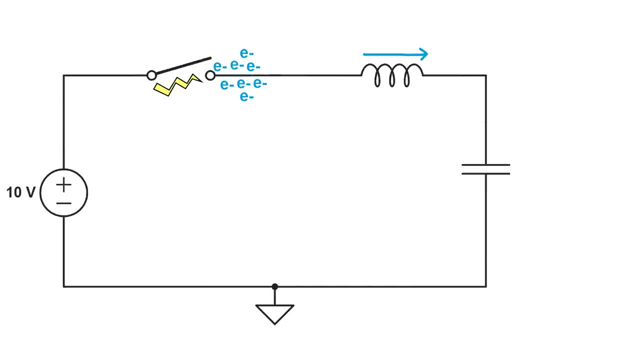 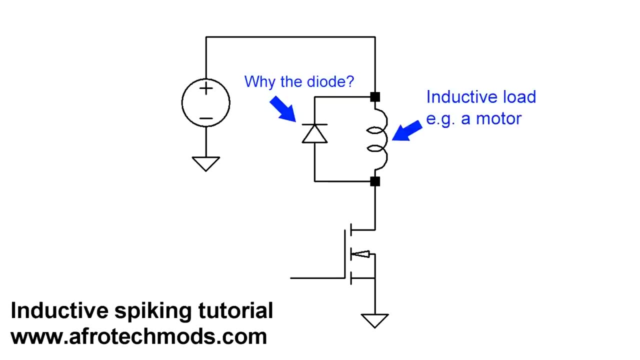 spike. This voltage spike can reach hundreds or even thousands of volts- enough to blow up any switch you connect here. If you want more detail about this phenomenon, check out my video on inductive spiking. In that video you'll learn that the solution to the problem is to add a diode. 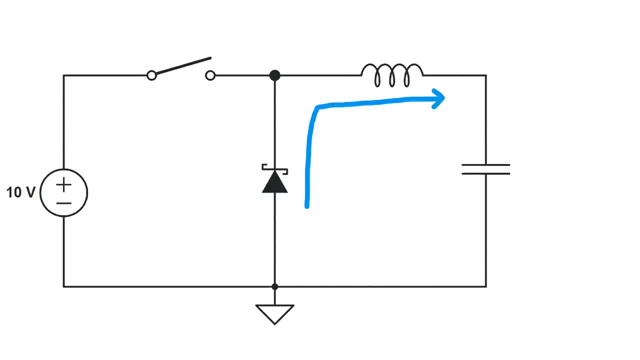 With the diode in place. now, whenever you open the switch, current can flow in a nice complete path and the voltage after the switch barely goes below zero. This is the classic buck converter configuration, and you can use this basic circuit to step high DC voltages down to lower DC voltages in a much more efficient way. 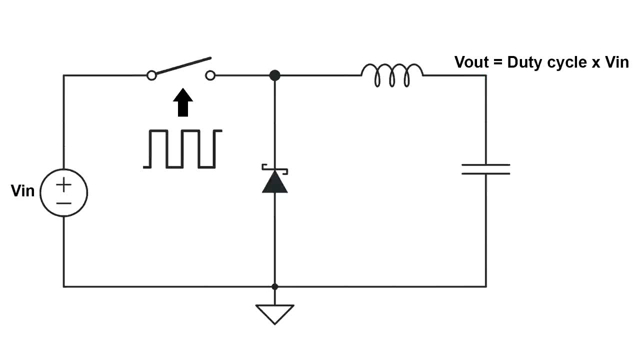 than linear regulators. Now in school they might tell you that this formula will give you the duty cycle you need to get the output voltage you want. Unfortunately, in the real world, this is garbage. As soon as you start drawing a few amps from your power supply, the various non-ideal parts, 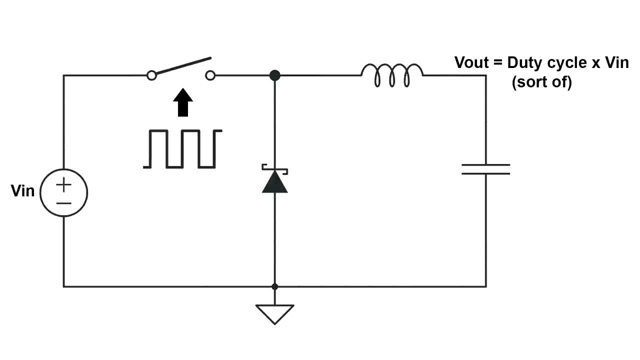 of the circuit will complicate things. You'll get power losses in your switch, your diode and your inductor, and even your wires. It's also highly unlikely that your output current will stay exactly the same. The more current your load draws, the more the voltage will drop. 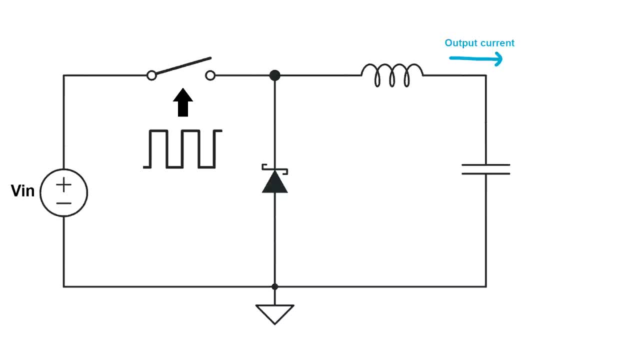 So what we need is a system that can continually monitor the output voltage and adjust the pulse width accordingly. If you draw more current on the output and the output voltage drops too low, increase the pulse width. If the output voltage gets too high, decrease the pulse width. 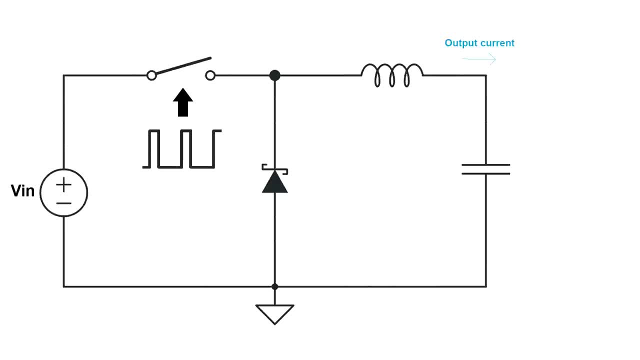 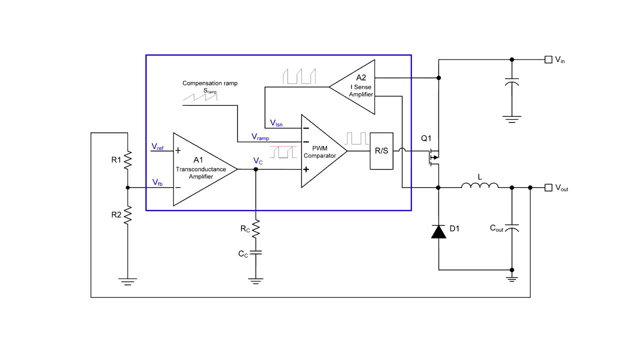 And we have to do this within a fraction of a second, otherwise we could fry the thing we're trying to power. In other words, we need a closed-loop control scheme with negative feedback. We can accomplish this by adding a feedback resistor network at the output: a ramp oscillator. 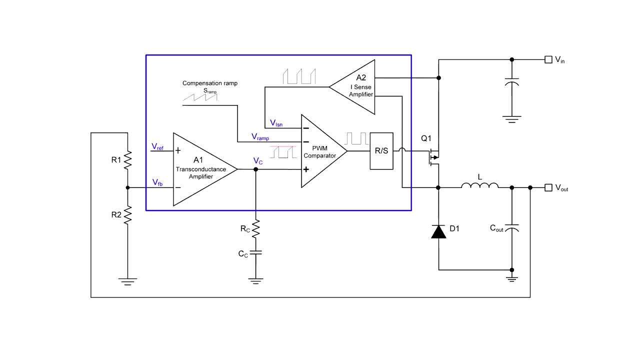 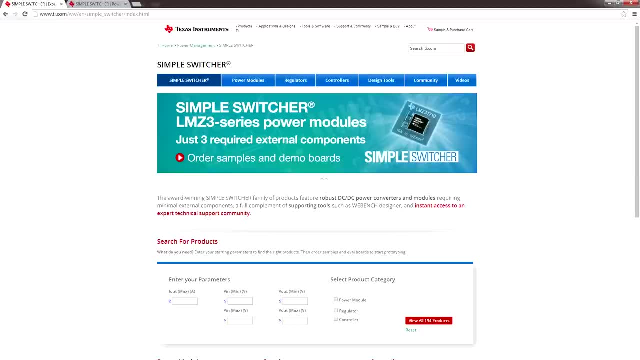 and an error amplifier. We're also going to need a precision voltage reference and a suitable slope comp- SHUT UP. Okay, how about we make things easy? Texas Instruments has a portfolio of products called Simple Switchers. All the Simple Switcher products are practically idiot-proof and all you have to do is add: 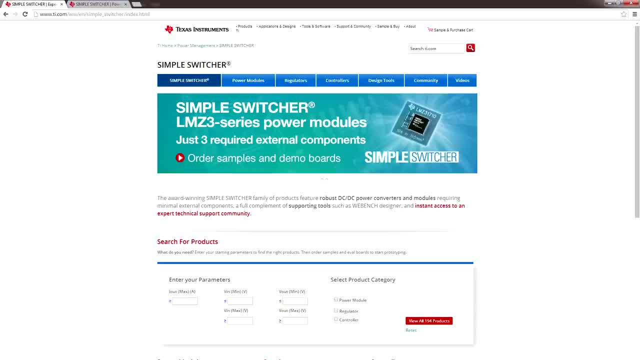 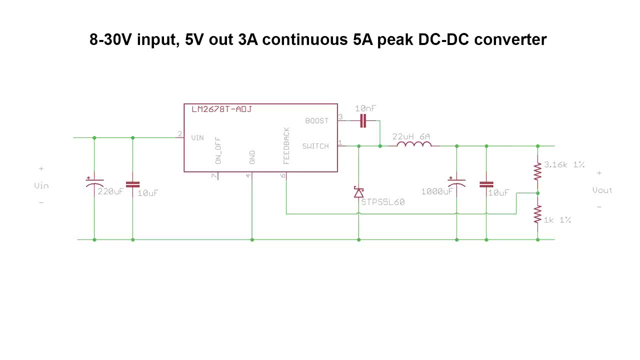 a diode, an inductor and a power supply. They take care of the complicated control electronics inside the chip. Let's use the adjustable version of the LM2678, and here's the circuit diagram. On the input, we have a large electrolytic capacitor in parallel with a ceramic capacitor. 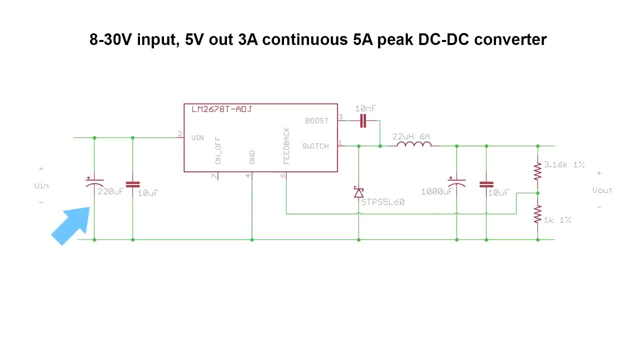 and this is necessary to ensure that the LM2678 can easily switch current from the input at very high speeds. If you don't have sufficient capacitance on the input, the parasitic inductance of your input power wires will be affected. This will limit the amount of current you can switch in every switching cycle and the 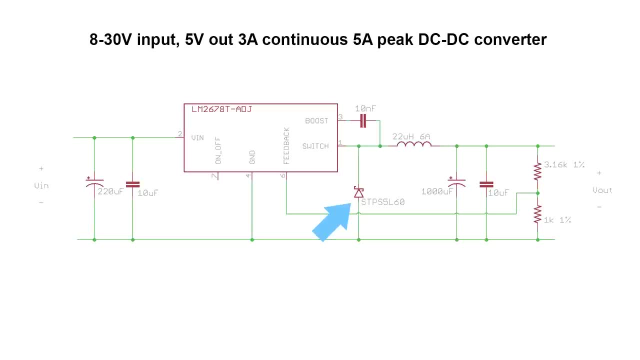 regulator just won't work For the diode. when you're designing switch mode power supplies, you almost always want to use Schottky diodes. These have a lower forward voltage than regular silicon diodes, so they produce less heat, which is something you always have to worry about when you're working with high currents. 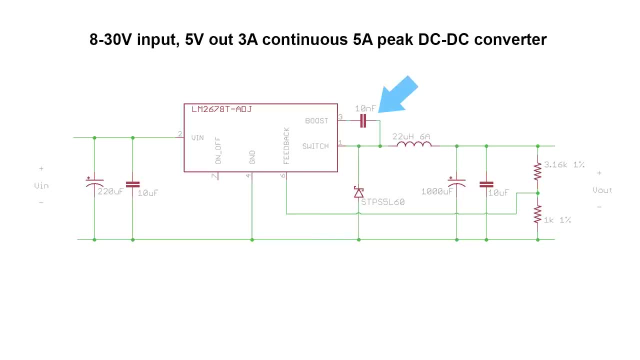 I'll put links to the components in the video description section. This is a bootstrap capacitor and it's used to help drive the switching transistor inside the LM2678.. It can be 10 to 100 nF and it should be a ceramic capacitor with at least a 50V rating. 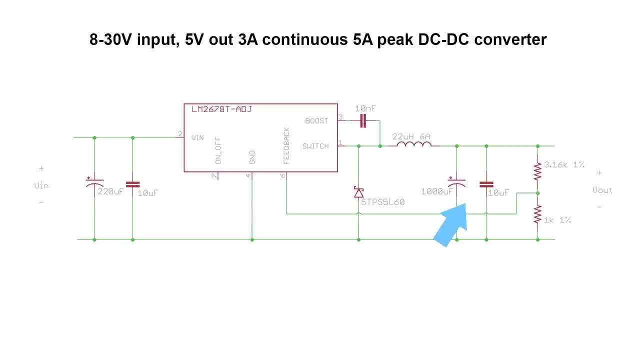 On the output. we have a combination of capacitors that will smooth out the high frequency content of the switching waveform, leaving you with relatively clean and stable DC. These resistors configure the LM2678 to give you a 5V output. Try to use 1% resistors if you want an accurate 5V output. 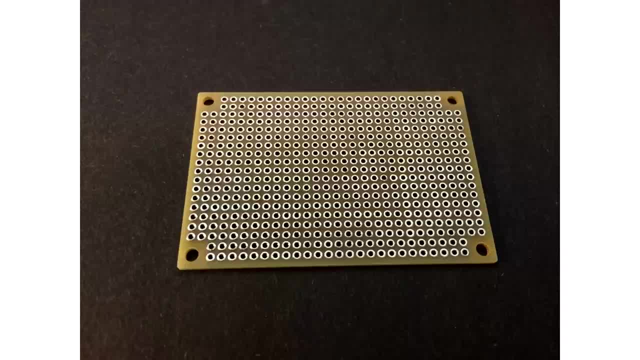 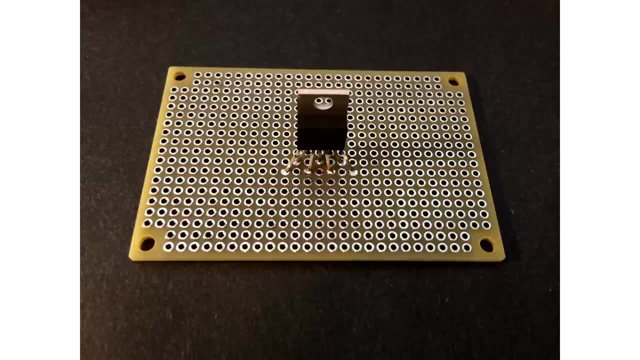 Alright, let's build this thing. Let's go, Let's build this thing. You don't want to use a breadboard for this. Use perfboard or make your own PCB Solder in the LM2678, first leaving a large amount of space around it to fit the other. 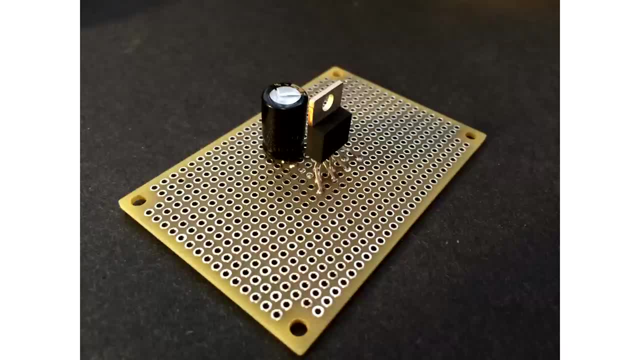 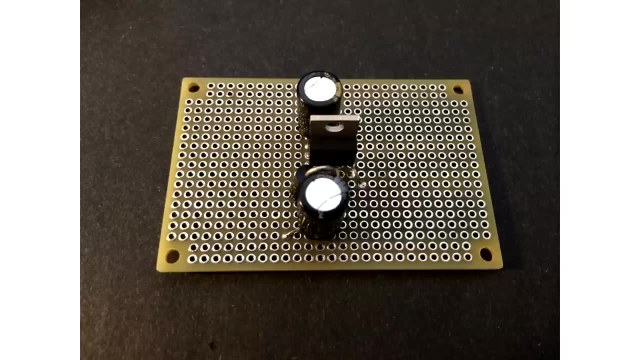 components. Solder in the input electrolytic capacitor within a centimeter or two of the controller and use short thick lines of solder to make the connections. Do the same with the diode and the output capacitor. Keep the component leads as short as possible. 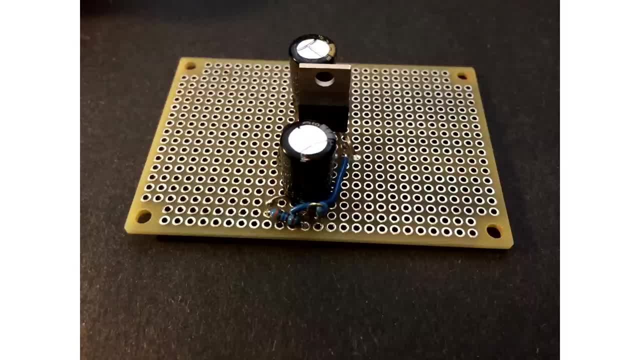 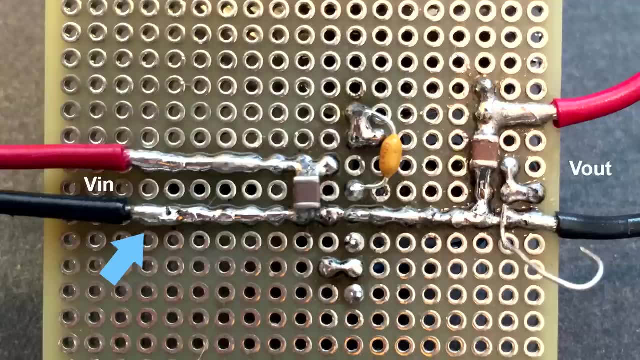 When you solder the feedback resistors, try to keep the wire going back to the chip as short as possible. The layout on the underside of the board is even more important than the top side. Notice how my ground is one continuous straight line and I arranged all the components on 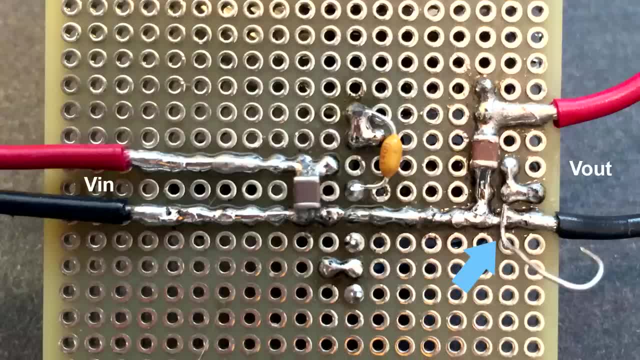 the top side around this. I also soldered on a ground wire for oscilloscope probing later. And look how I soldered the ceramic input and boost capacitors directly across the pins of the LM2678.. You can see the difference between the two. 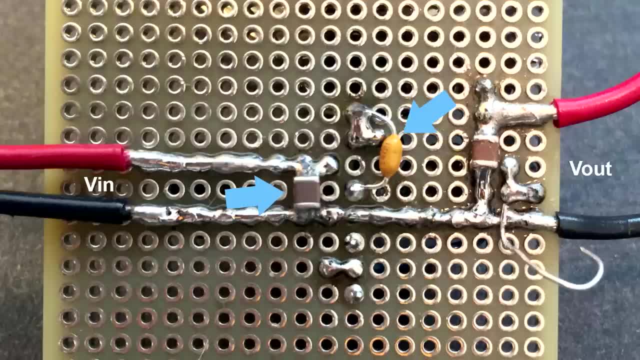 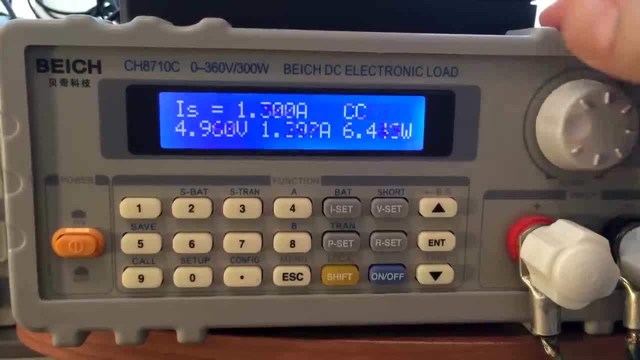 It's a great idea. The caps are even a few millimeters away from the chip. Everything will perform a lot worse. OK, now that everything's soldered up, I'm going to power my buck converter with 10 volts and I'm going to use my programmable electronic load to see how it performs, delivering different. 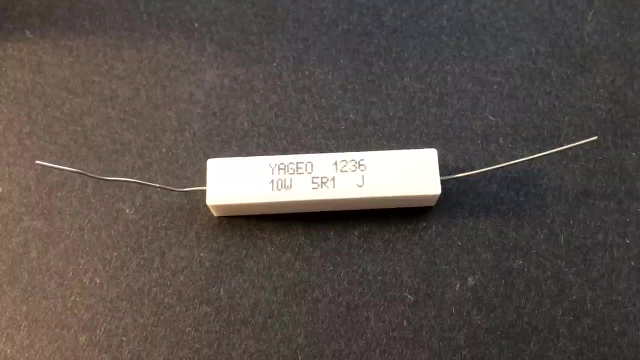 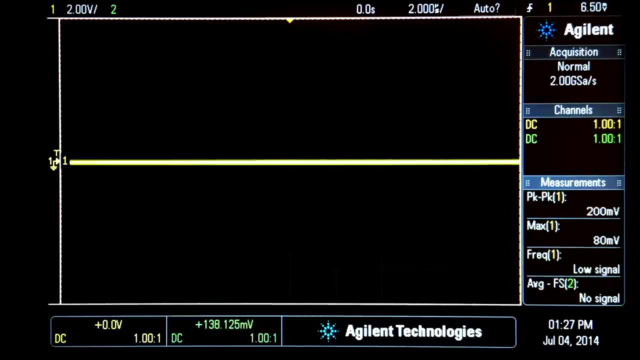 amounts of current. If you're doing this at home, you can just use 5 ohm, 10 watt power resistors as a dummy load. First, let's check the output voltage. is what we want it to be And it is. 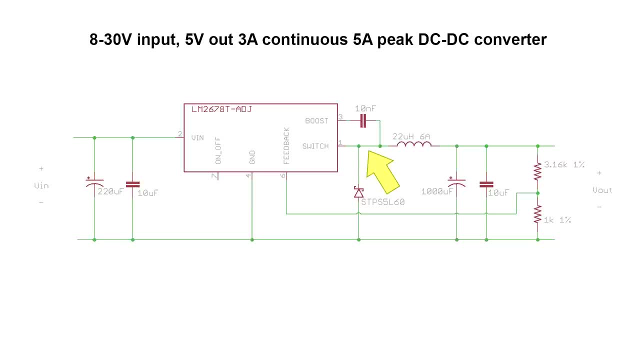 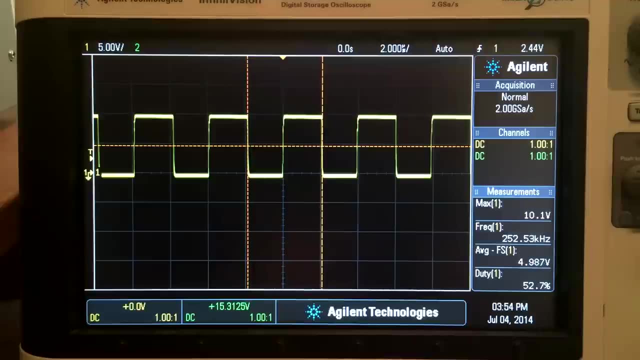 Perfect, 5 volts DC. Now let's take a look at this node in the circuit, which is called the switching node. This is before the LC low pass filter. You can see our familiar 0 to 10 volt square wave and the switching frequency is 250 kilohertz. 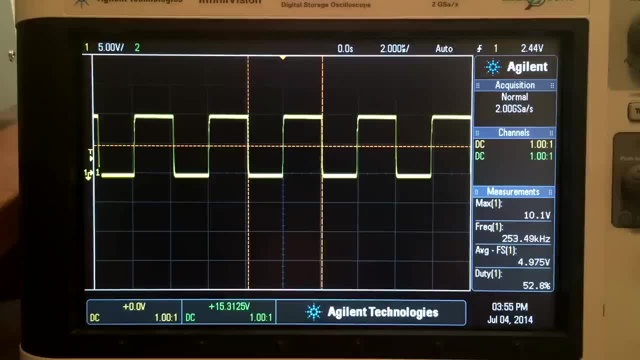 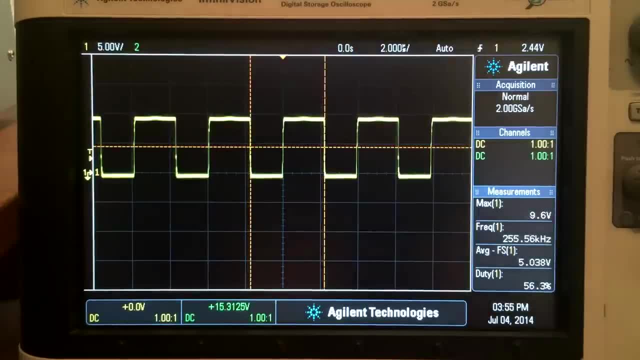 But you can see the duty cycle is about 52% instead of the theoretical 50%. This is with a half amp load on the supply. If I increase the load to 3 amps, the duty cycle increases to 56%, And at 5 amps the duty cycle increases to 56%. 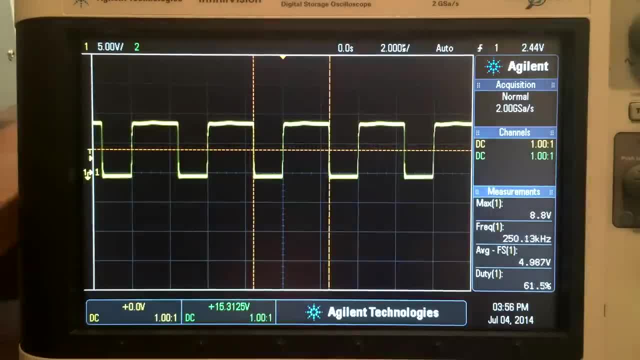 And if I increase the load to 3 amps, the duty cycle increases to 56%. And at 5 amps the duty cycle increases to 56%. And if I increase the load to 3 amps, the power losses are significant enough that 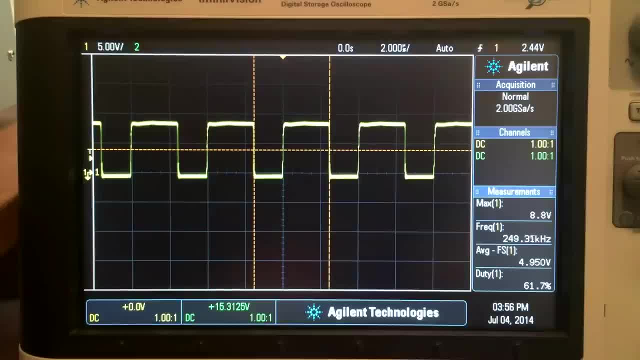 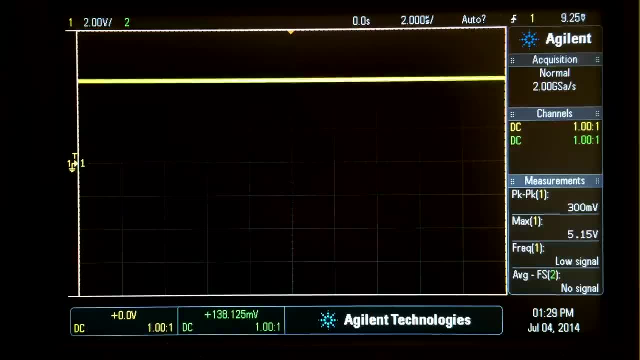 the controller had to change the duty cycle to 61% to maintain the regulated 5 volt output. Remember when I said we were getting a perfect 5 volts? I LIED. Let's change the coupling on the oscilloscope to AC coupling and zoom in. 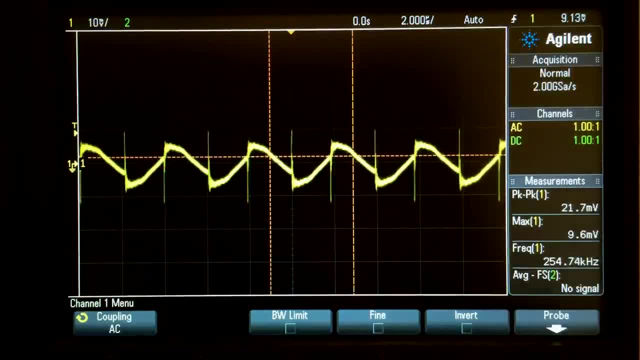 You can see that there's a small AC component on the output because our low pass filter isn't perfect. We call this the output ripple of the power supply because it looks like little wicks, but it's not. It's actually a little more than that, because it looks like little wave ripples. 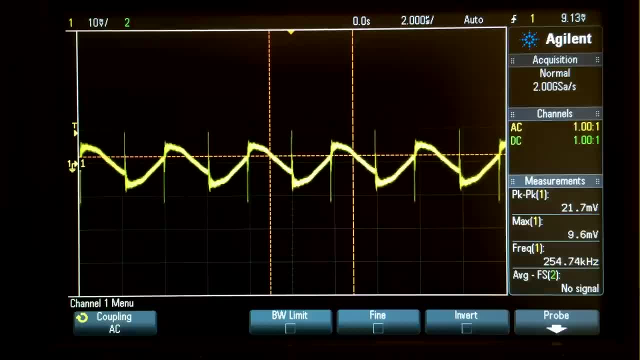 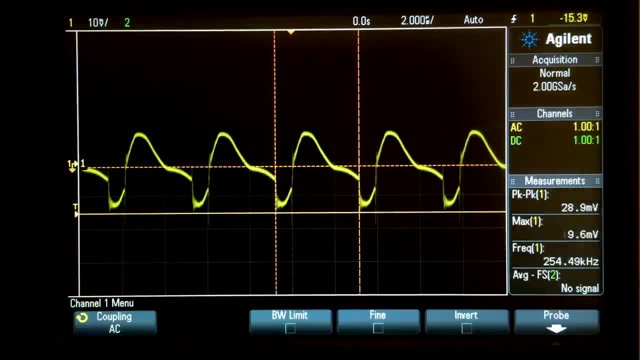 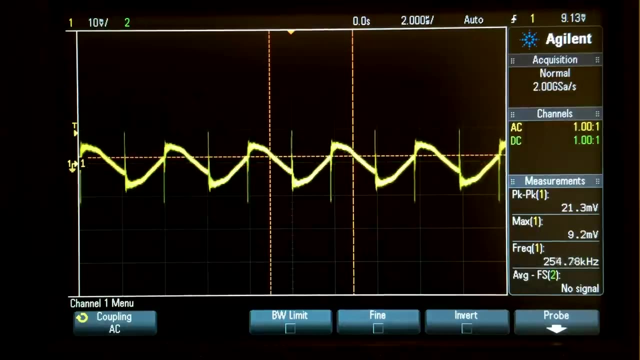 We have about 20 millivolts of ripple and noise with a 3 amp load. If I increase the load to 5 amps, things get noisier. If I increase the input voltage to 28 volts, the ripple waveform gets bigger and it changes. 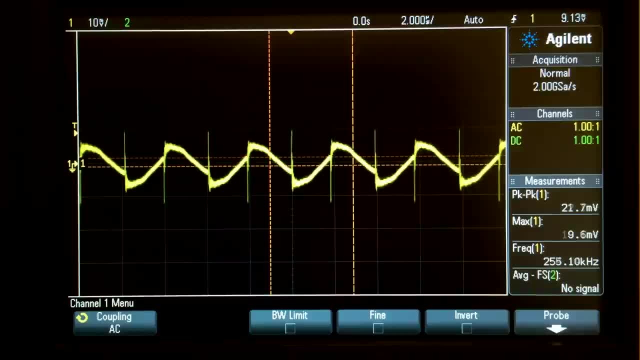 shape. Ideally we want this ripple to be as small as possible. For most applications under 100 millivolts, peak-to-peak will be fine, But in general you don't want to use switch mode power supplies to power sensitive circuits. 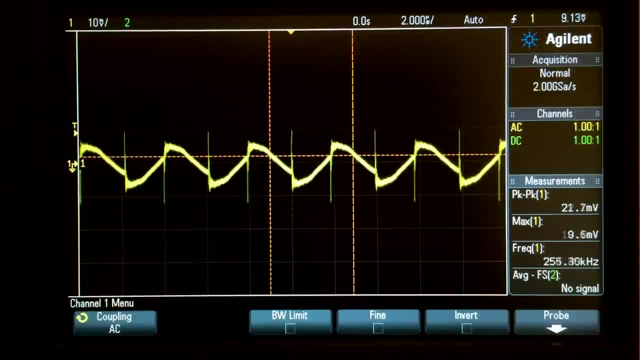 This makes it difficult to control the power in the power supply and it's not safe for most applications to control it. The only things that are different is that the output voltage on the output is too small. positive circuits like radio receivers. If you want to learn more about measuring power supply, ripple enable video annotations. 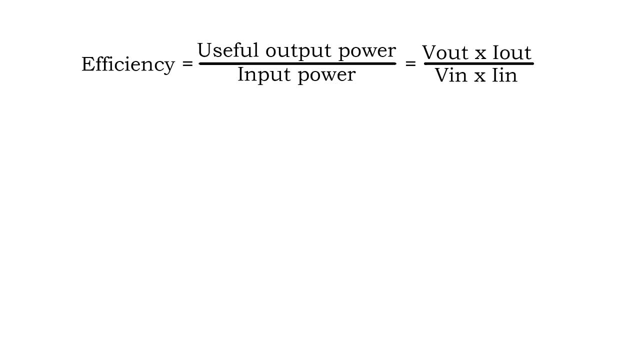 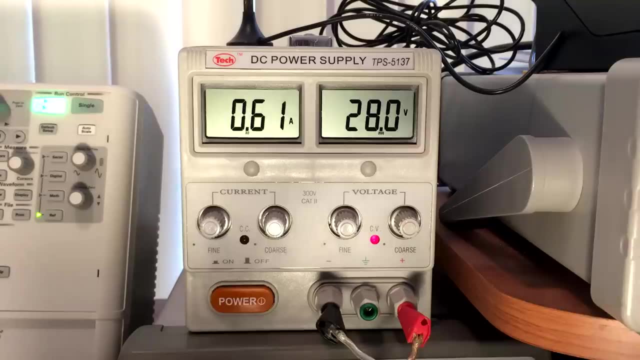 and check out Dave Jones' excellent video on the subject. Now let's measure the efficiency of our supply and compare it to a linear voltage regulator. From a 28 volt input, my bench power supply is supplying 0.61 amps to our DC-to-DC converter. My multimeter says the output of the converter is 5.019 volts and I have the load set to exactly 3 amps. If you're doing this at home with resistors as a load, make sure you use your multimeter to accurately measure the output current. 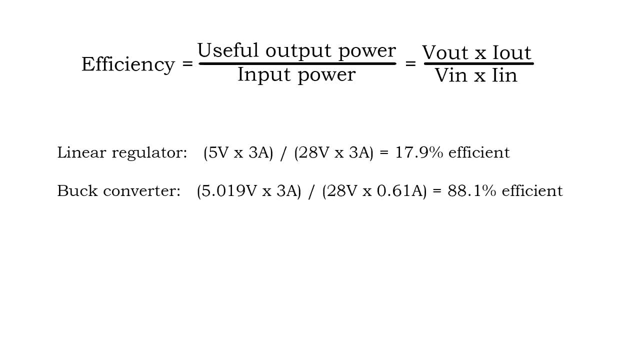 Here's the equation for power supply efficiency. Plugging in the values we measured earlier, we find that our power supply is around 88% efficient, which is pretty good. This is why people usually use switch mode power supplies for currents higher than 1. 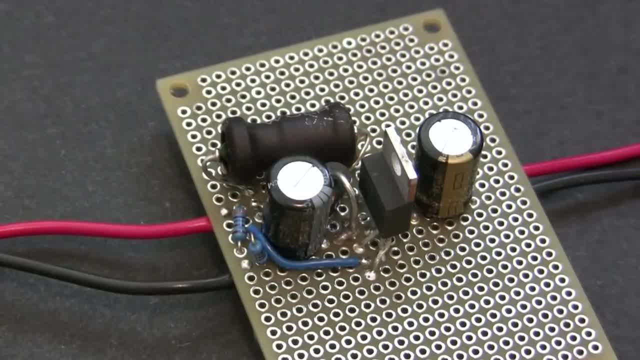 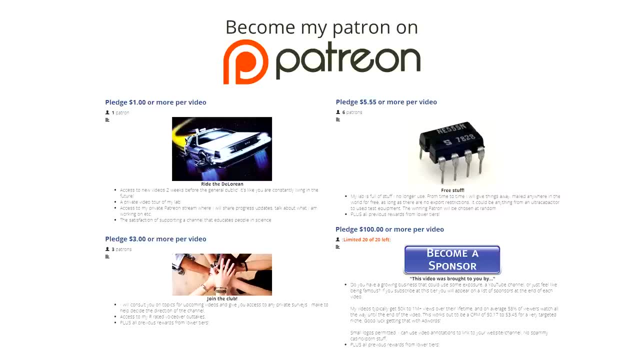 amp. Alright, now you know how to make a high current power supply, and knowing is half the battle. Thank you for watching and if you liked this video, please check out the video description section to see how you can support me. Make sure you check out Patreon, which is kind of like an ongoing Kickstarter campaign. to help fund the channel. 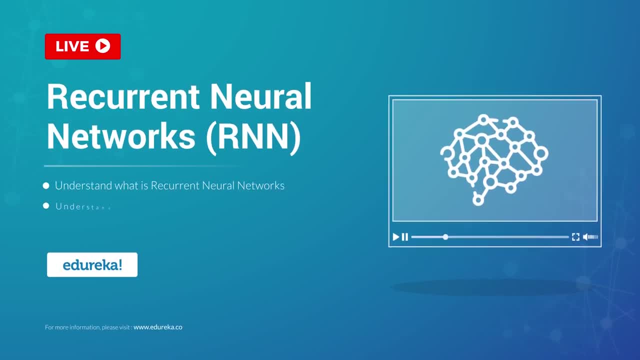 Hello everyone, this is Saurav from Edureka, and today we'll be focusing on recurrent neural networks. So, without any further ado, let us move forward and have a look at the agenda for today. So we'll begin by understanding why can't we use feedforward networks for